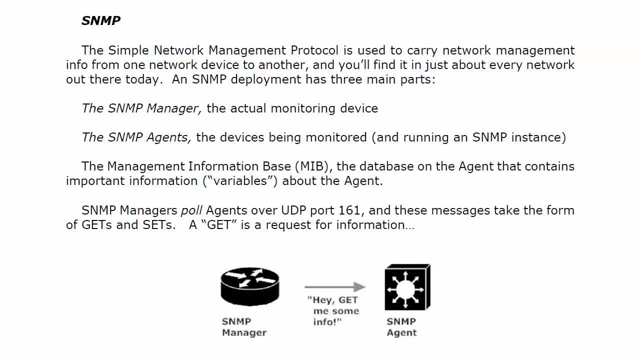 explanations about this. I've seen some confusing explanations about this. I've seen some confusing explanations about this. I've seen some confusing explanations of these over the years. So this is about as straightforward as it gets. A get is a request for information, And I've 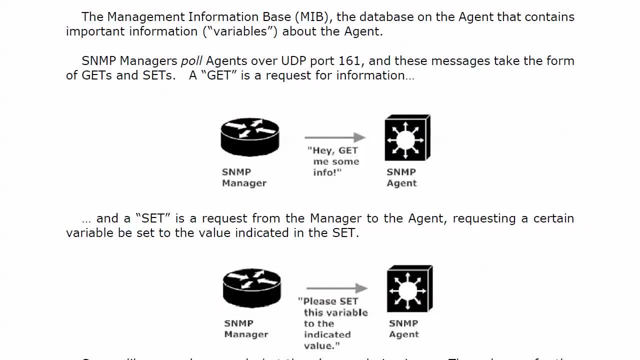 always remembered. hey, get me some information. It's a get, Tell me something. Then you have a set, which is where the manager says: I would like you to please set this variable to the value I have indicated here. A get is a little ruder than a set, but these are Gegett. 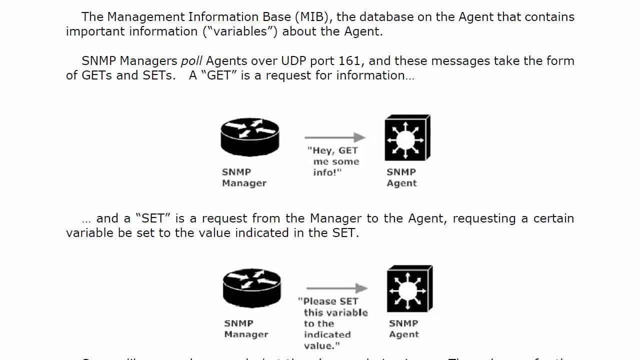 the two main forms: a communication between manager and agent. problem here. And if you don't, there's a hint in the arrows Because you'll notice those are one-way communications- Manager talking to agent, manager talking to agent, And the problem is. 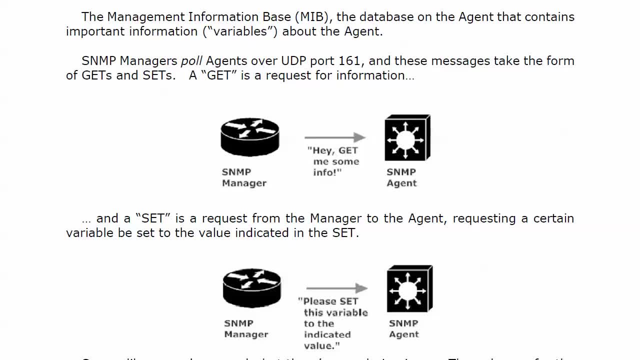 let's say that you have a 10-minute interval set on this polling And 10 seconds after the most recent polling some variable changes wildly on the agent. Something happens, an event occurs that the manager really should know about right now. Well, with gets and sets you don't have that. 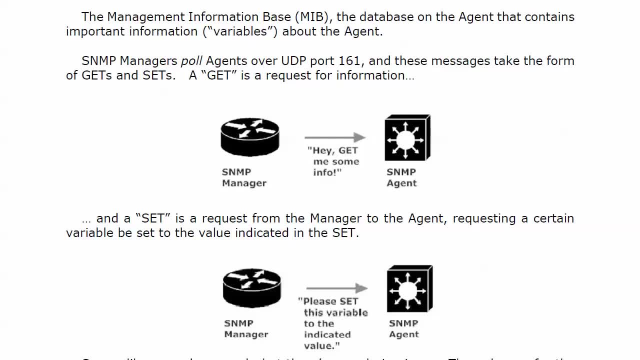 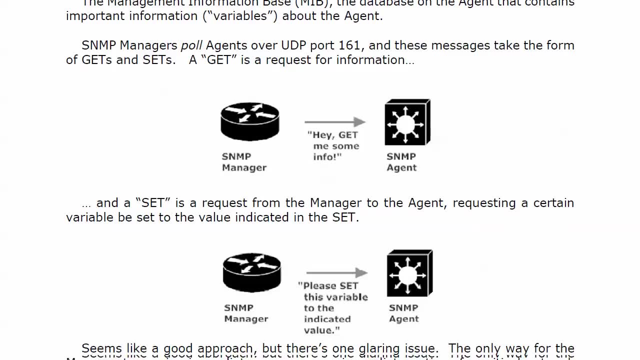 And then the next time the manager asks, hey, get me some information, it could be: hey, nine minutes and 50 seconds ago something really bad happened. That's not the kind of rapid notification we like in today's networks. So to get such a quick notification on an event, 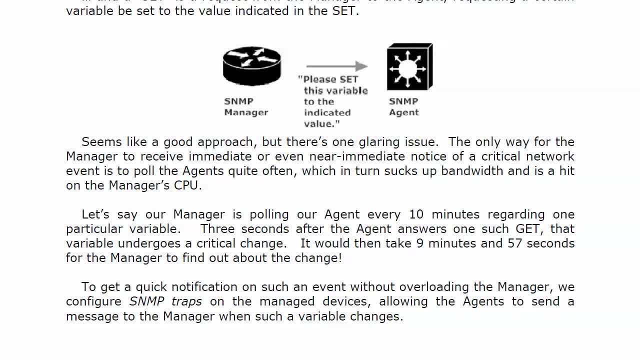 without overloading the manager by over-polling, because one approach you could take is: well, we'll just poll every 10 seconds. That's probably not good either, because you're putting a huge workload on the manager. the agents have to answer all those pollings and there could be a little bit of a bandwidth. 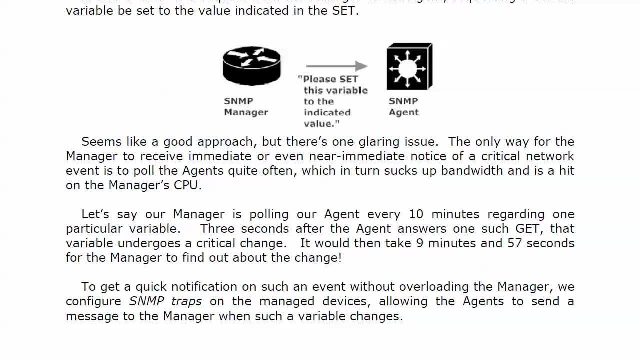 issue in there, But I'd be more worried about the overload on that manager. What we can do instead is configure what we call a trap. Yes, it's a trap, And I'm really bad at it. Do your own. We configure these traps on the managed devices and it allows the agents to send a message to. 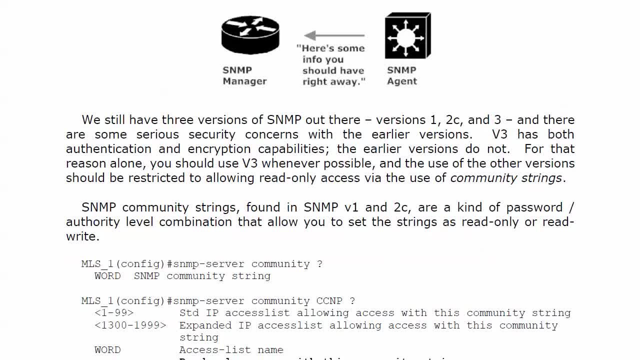 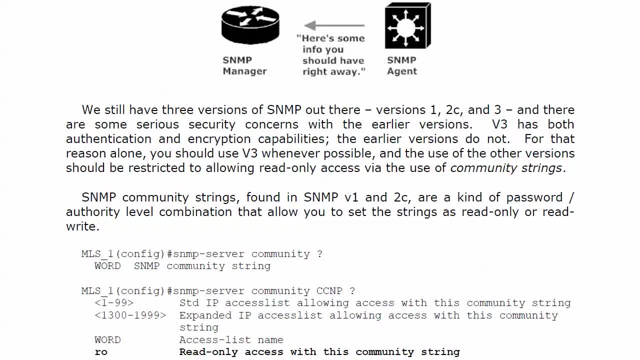 the manager. when such a variable changes, It's like: here's some information that you should have right away Now. we still have three versions of SNMP out there- Versions 1, 2C and 3. And we know that's fertile ground for exam questions. But also you need to know these: 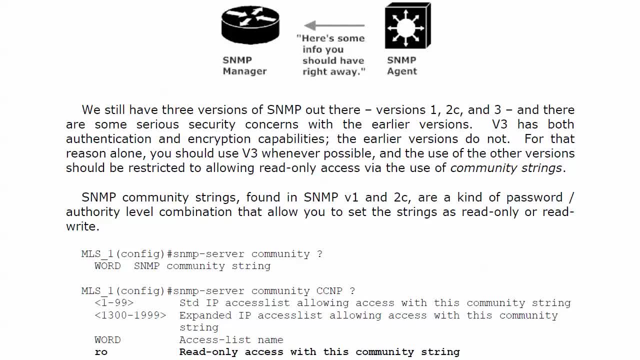 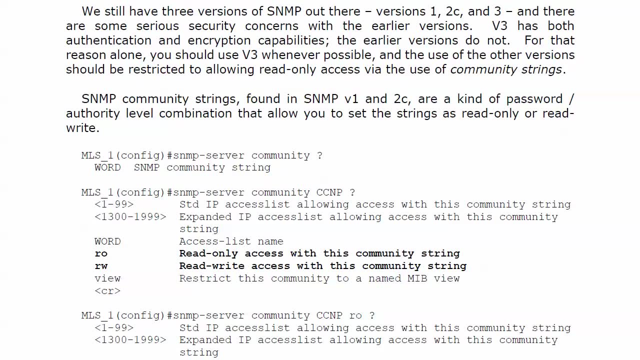 differences for your work with production networks, because there are serious security concerns with the earlier versions. Version 3 has both authentication and encryption capabilities. The earlier versions do not. So whenever possible, whenever possible, you should use version 3.. The use of other versions should be restricted to. 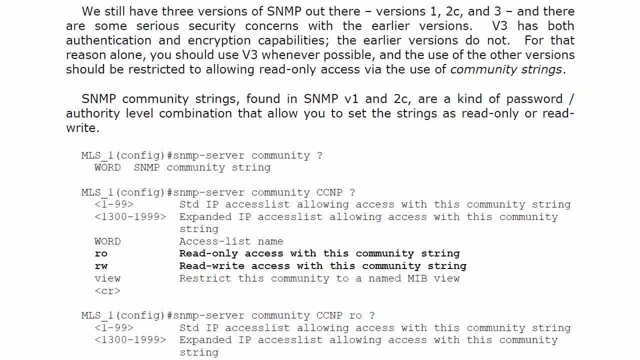 allowing read-only access via the use of a community string. I love that It's a community string. Well, what the heck is a community string? It's a kind of combination of a password and an authority level that are found in the first two versions of SNMP that allow you to set strings. 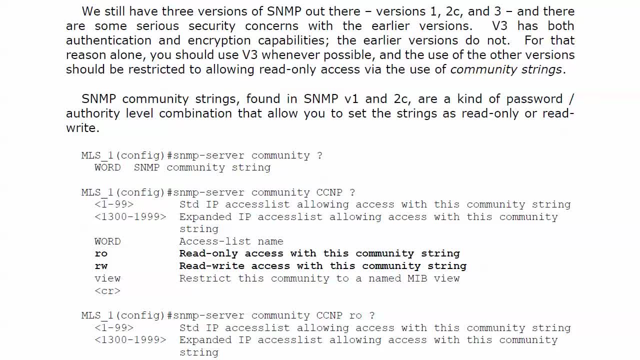 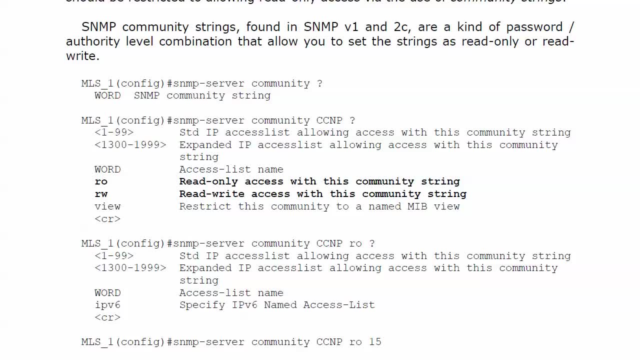 as read-only or read-write And I've got one of these for you on the board and I can walk through this on the live equipment. We are going to do a little bit of version 3 there, But you can see the name is simply SNMP server community or the commandos. You follow that by. 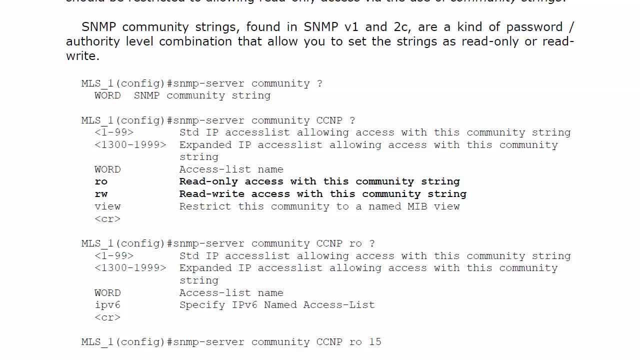 the name of the community string that you're creating. Then you've got a couple of options and the important ones, the more important ones in my humble opinion, are RO and RW, which is read-only and read-write. You can type in ACL into it and then you end up with the 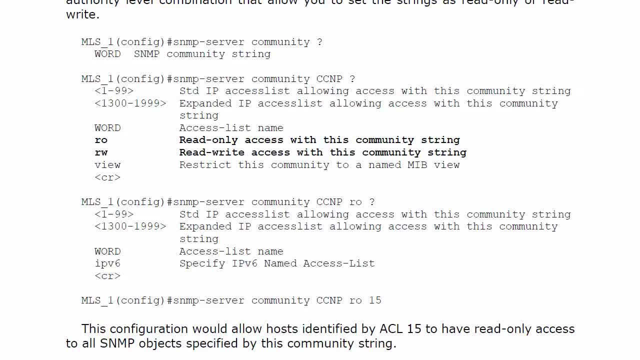 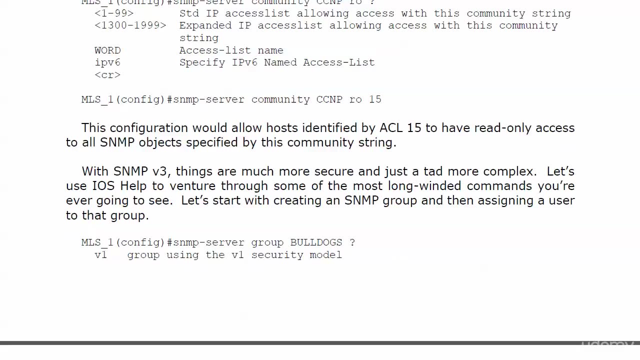 host, And this would allow hosts identified by ACL 15 to have read-only access to any SNMP objects that are specified by this community string. This was fine for a long time, but again, the lack of encryption and authentication. we're not real crazy about that, So thankfully version 3 came. 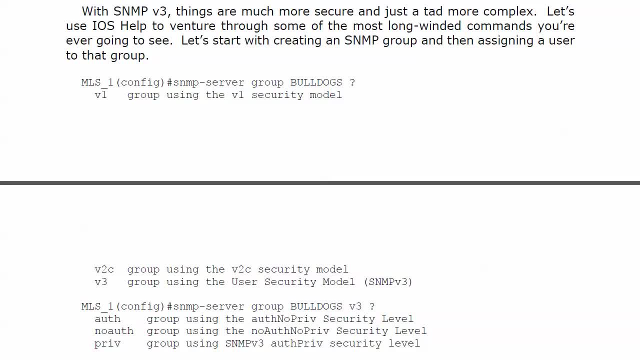 along and we're going to look at some of this on the board and go through iOS help And you are going to see some of the most long-winded-to-disk commands you are ever going to see- Long-winded, indeed, I guarantee you. we're going to see that magic dollar sign because the commands 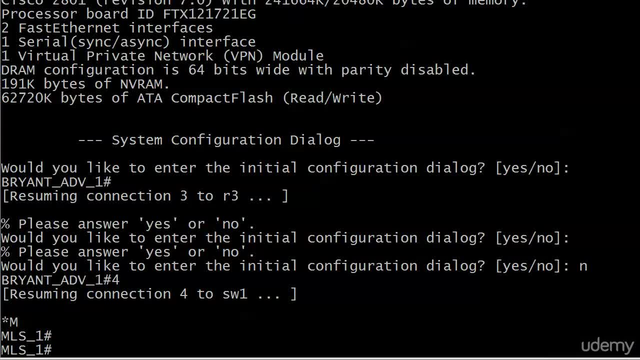 get so long on this one. So let's go ahead and start. First off, we're going to create a group, then you create a user and then you define the location for traps. That's basically the three steps we're going to do here, And let's go ahead and dive in with that group command. Let's do that. 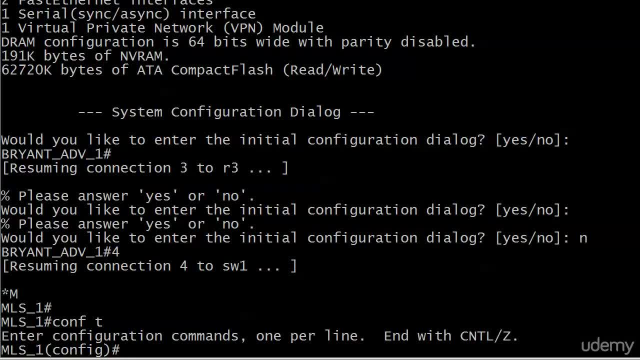 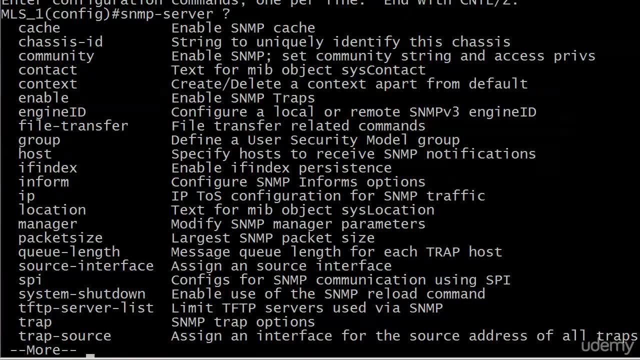 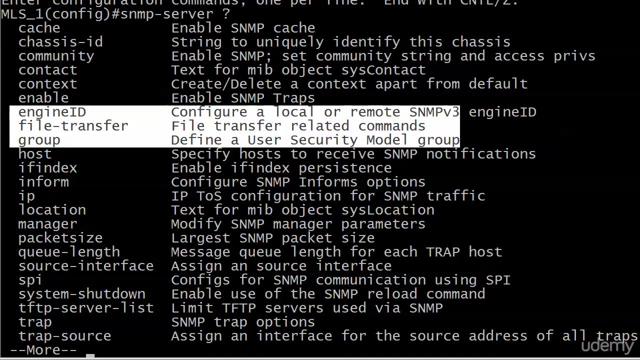 first, No use in creating a user with a group association if the group hasn't been created yet. So SNMP server- you need that little hyphen there. A lot of options here, too, but only a few that we really need, And the one we need right now is group. We are doing what is officially known as 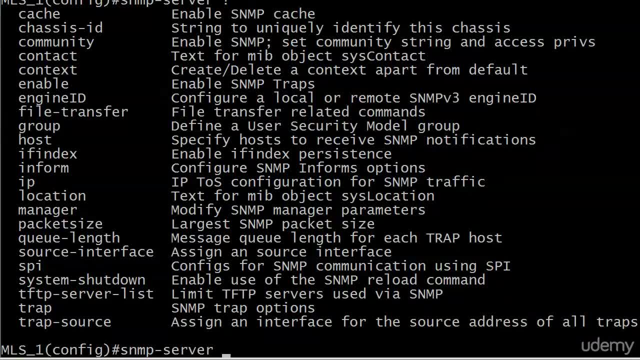 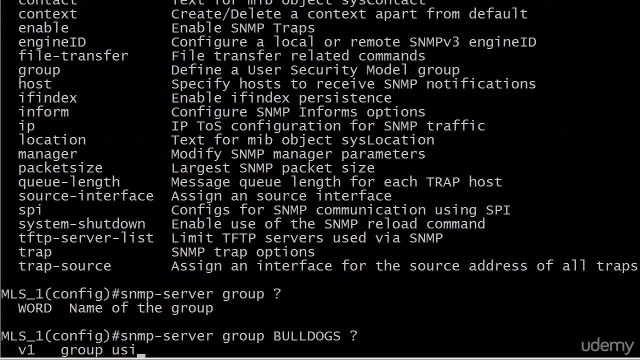 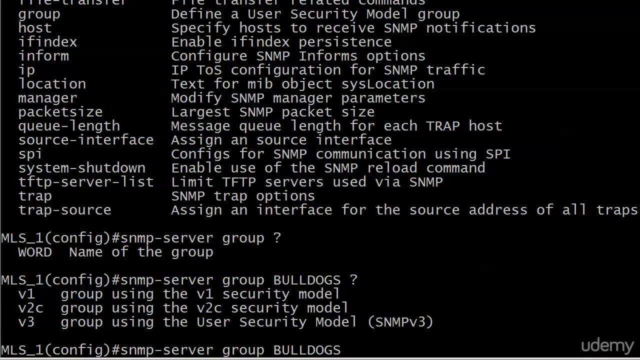 defining a user security model group. So let's get the heck out of that. And we've got the word group. Then you put the name of the group And here comes the first part. that really tests whether you understand which versions have authentication and authentication. So let's go ahead and do that. 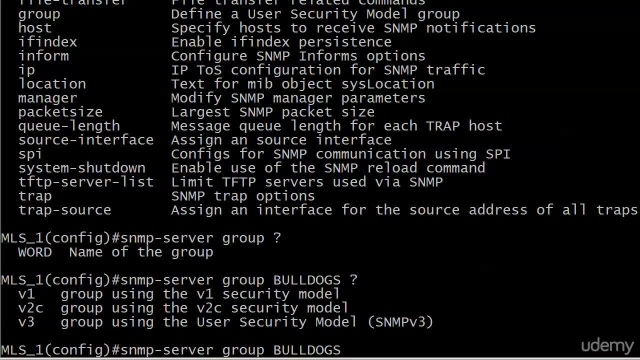 Because you've got to pick one of these groups And we're told version 1 uses the v1 security model, Version 2c uses the 2c security model And then finally, version 3 uses the user security model, version 3.. Not a lot of detail given here about what those first two security models are. We know. 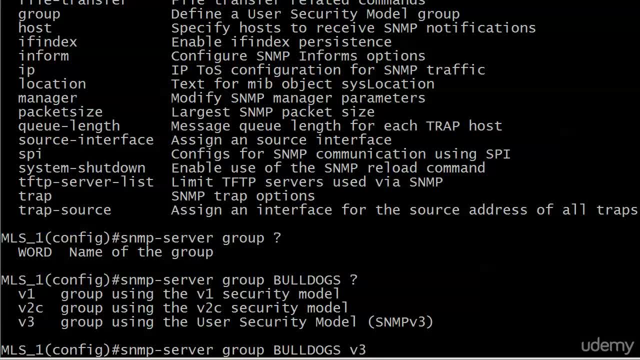 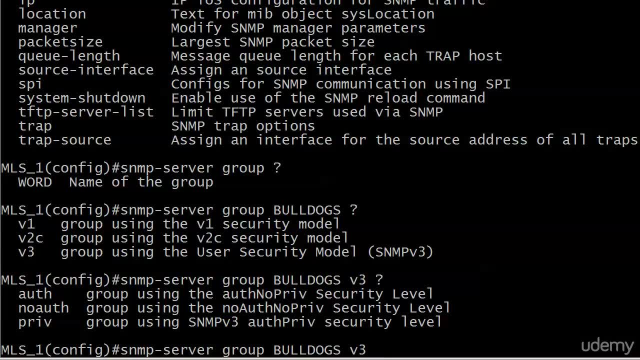 what they are. so we're going to avoid them And we're going to choose v3.. And here comes the second test of whether you studied or not. right, We have to know what these levels are, And they look really odd. You know you've got capital letters in the middle, which always makes things. 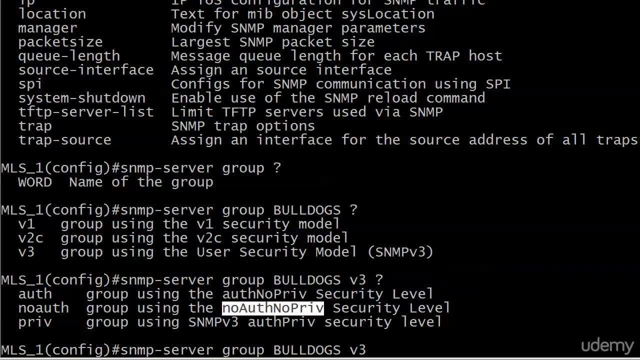 look strange: You've got auth no priv, no auth no priv and auth priv, Hmm, okay. Well, if we break those down, though, what we're talking about is authentication and privacy, And the privacy part comes in with encryption. So, with these particular groups, what we have is a group that has 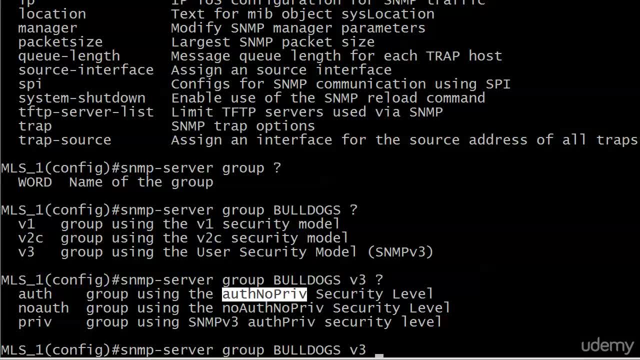 authentication but no privacy, meaning it has no encryption. You have another group that has nothing. It has no authentication and no privacy, And then, finally, we have a group that has both authentication and privacy. So that will be no surprise to you. That's the one we're going to go with. So we need to put priv there And what else. 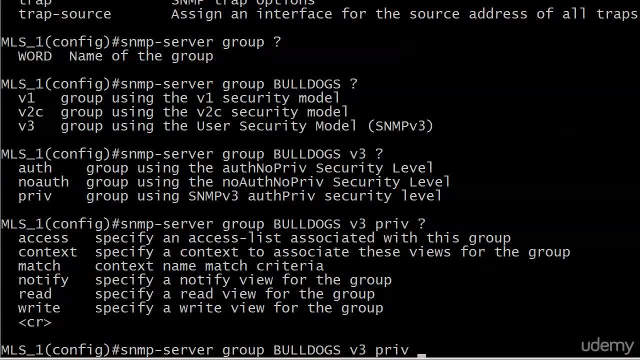 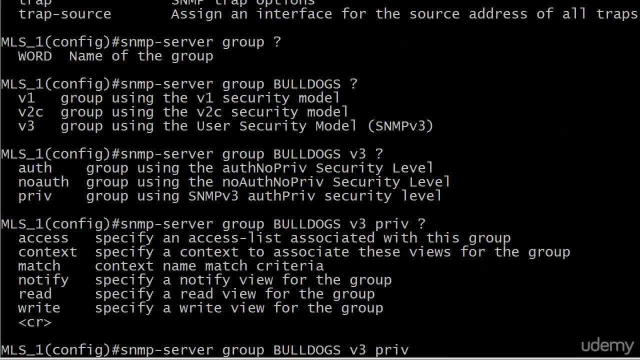 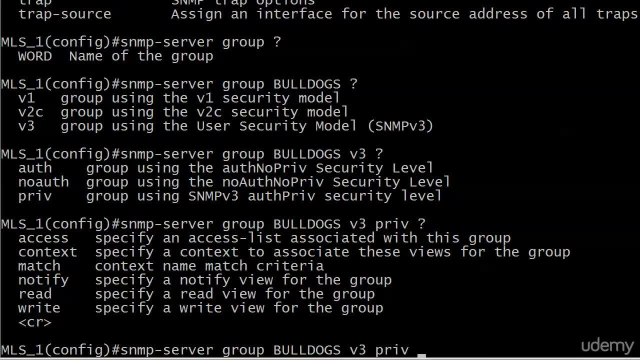 do want to tell you a couple of things you need to know about these groups: notify, read and write. If you don't define a read view, all objects can be read. Okay, Makes sense. If no write view is defined, no object can be written. And if no notify view is defined, 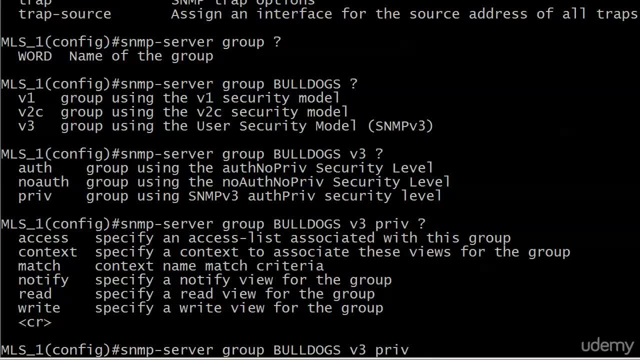 the members of the group will not be notified of changes, which makes sense too. So watch that read-write thing because, again, the read view. if you don't create a read view, everything can be read. If you don't create a write view, nothing can be written. So that's about it for those. Now. 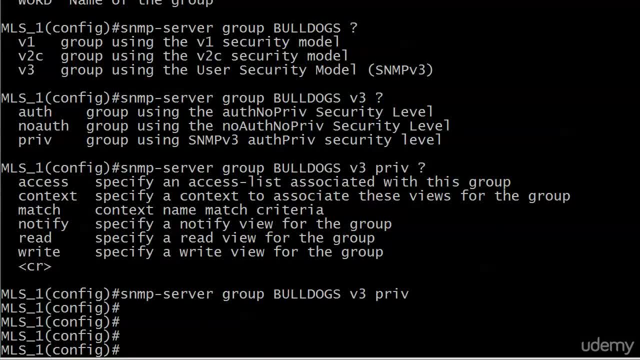 we're just going to go with that right there, and that creates our group. And you're saying: well, Chris, that wasn't long-winded at all. Stick around, Don't go on any long trips. We got one for you here. Let's see, We've got SNMP server and we're going to go with user and we're going to 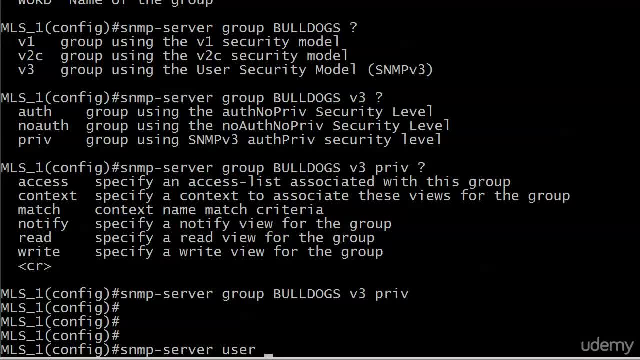 use SHA for authentication and AES 182-bit. Let's go with 128-bit encryption. We'll see those choices as we go along. And one question that may well have come to your mind when we were talking about the security levels. you know why would you ever choose a lesser security level? You would always. 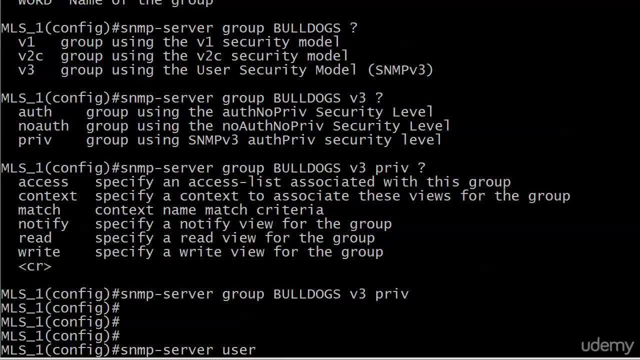 choose auth-prevenless for some reason. The only reason I can think of is that your hardware wouldn't allow it or you thought you didn't need it. Now, some of these choices here with SHA authentication and AES encryption: it's going to be dependent on your hardware whether you can actually run those or not, But that's what we're. 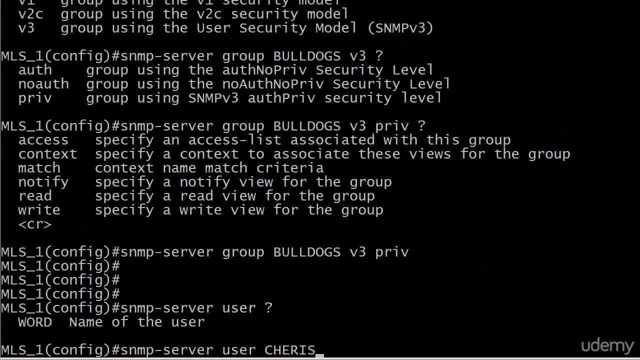 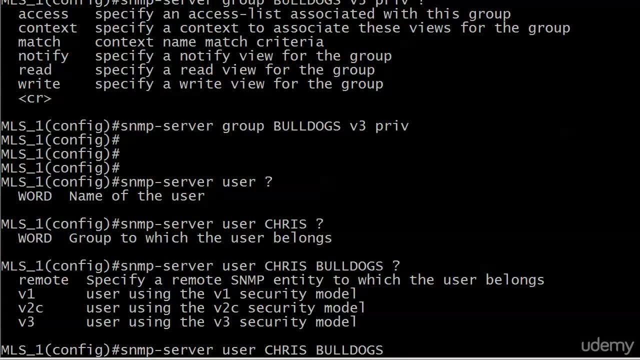 going to go with here. So let's see what we've got for user. First off, we'll put me in And group to which the user belongs. We know that's Bulldogs. And now we've got remote, and then we have security models again, So we're going to stick with V3.. Then we have access, auth and encrypted. 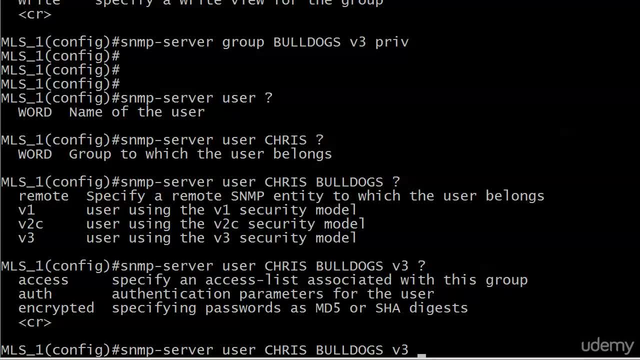 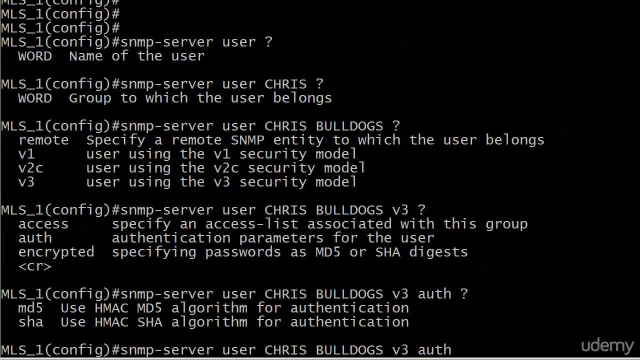 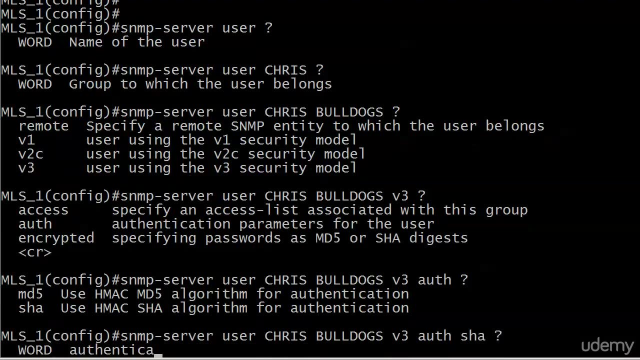 whether we're specifying passwords as MD5 or SHA. So tell you what? let's go with auth here, And the choices are MD5 and SHA. and, all things being equal, if your hardware can handle it, it's not even a choice. You're going to go with SHA here. Then we've got the authentication password for user. Notice they. 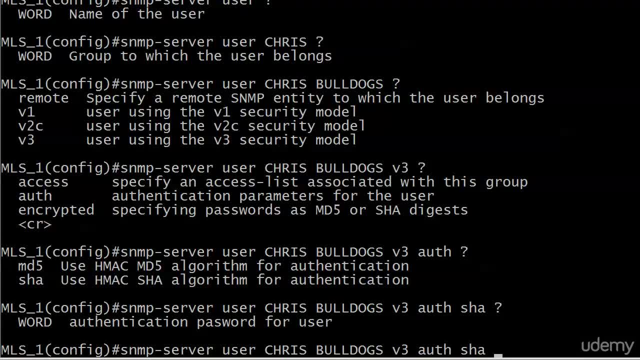 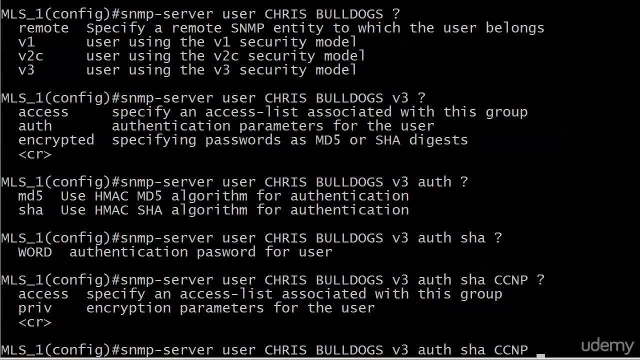 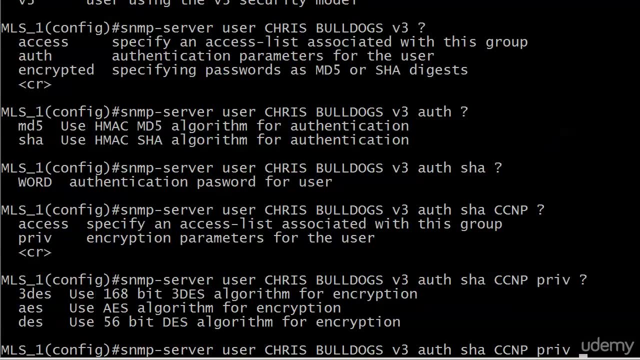 misspelled password. So let's see, we'll go with CCMP for that password. Then we've got our access and priv levels And we're going to go with priv for encryption parameters for this user, Because that's where AES and 3DES and DES. 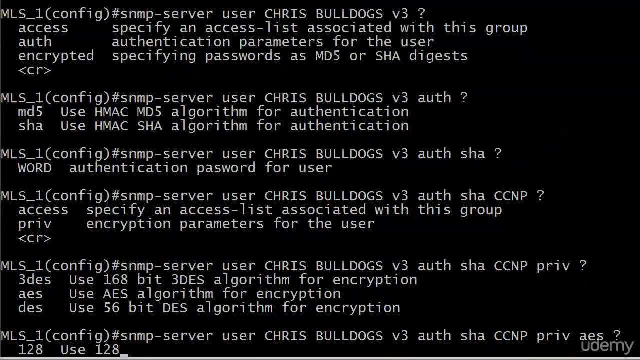 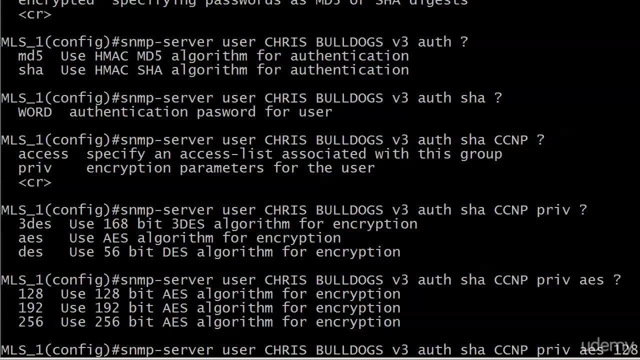 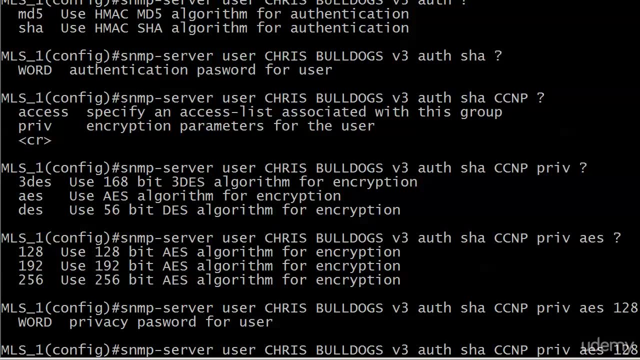 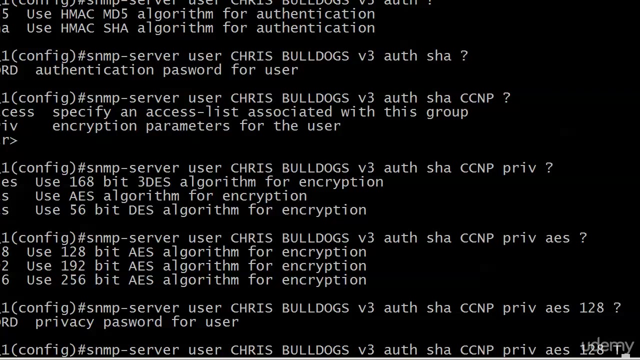 are hiding, So we'll use AES. And then, finally, how many bits do you want with that, Mr Wall? I'll take 128.. And we have to continue, because now I've got to enter a privacy password- 1s for user, And even I, at this point, am tired. 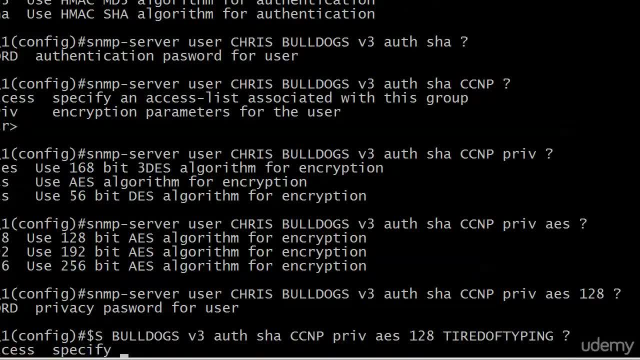 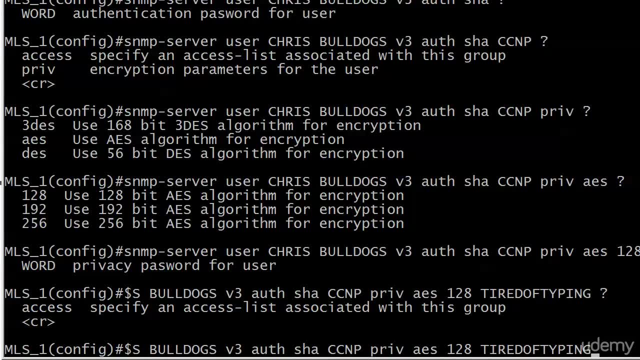 of typing. so I will put that in for my privacy password And I can still associate an ACL with this group. But I am going to just leave it right there and also get rid of that null space. Watch that at the end, And in case you've never. 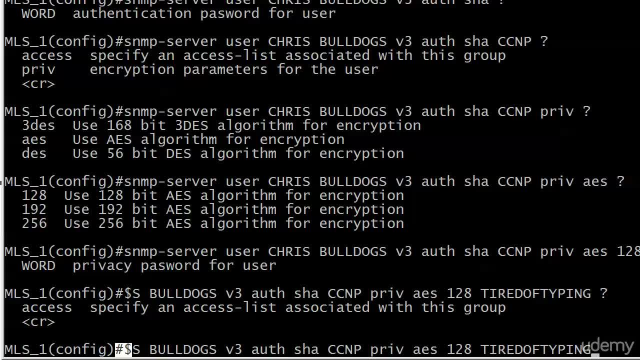 this odd prompt before. when you get a dollar sign here, that just means that your command is too long to be displayed on the line and full. if you wanted to start it at the beginning, see it from the beginning, you could just go ctrl a and that will move your cursor to the front and also move the 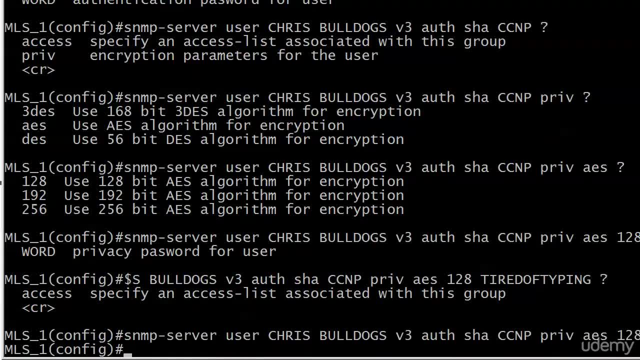 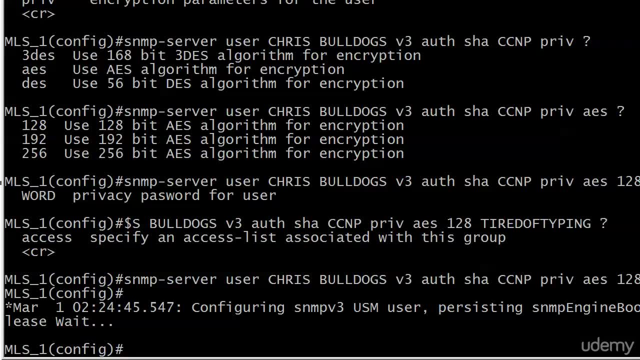 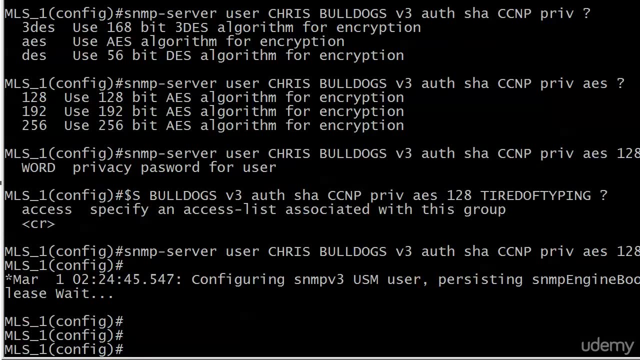 command to the front. so that is it for that command. now we need to define the location for traps and you'll notice it mentioned configuring snmp version 3, usm, user, persisting, etc. and then please wait. and then we're done so. so far, so good. now you just simply have to define the location. 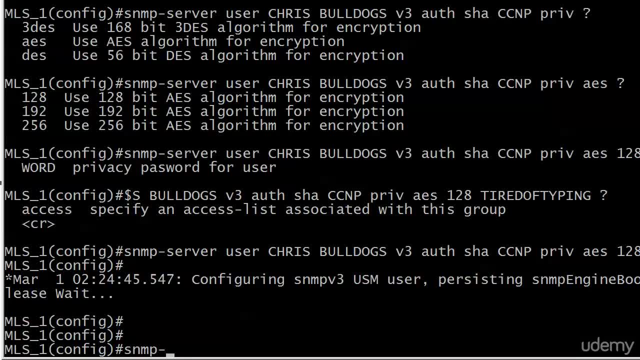 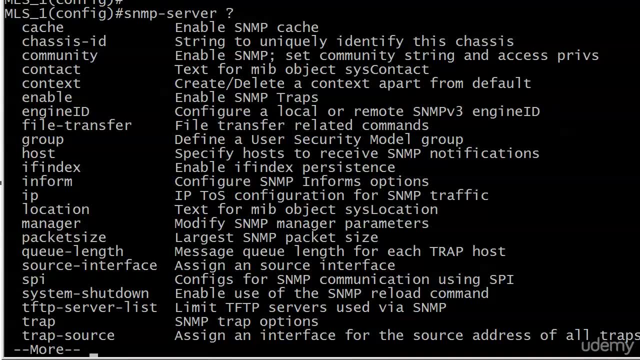 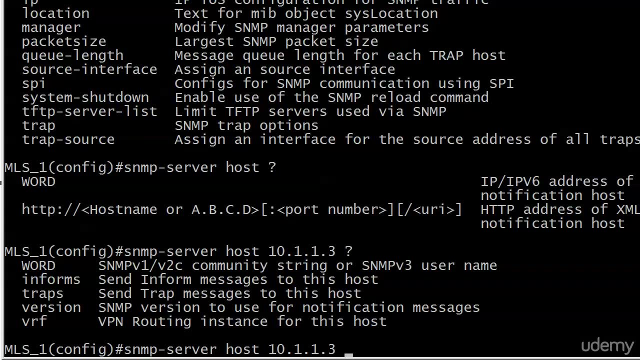 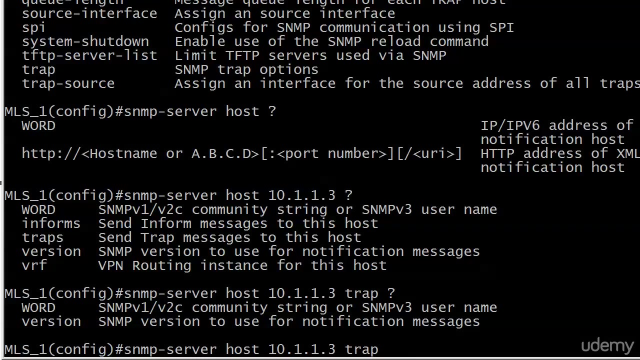 for traps, or is it that simple? let's, let's use the command, and this time we want host- specify host- to receive snmp notifications, and then we're going to put 10, 1, 1, 3 in for this one and we're asked for a couple things. what we want is to send trap messages to this user. then you've.